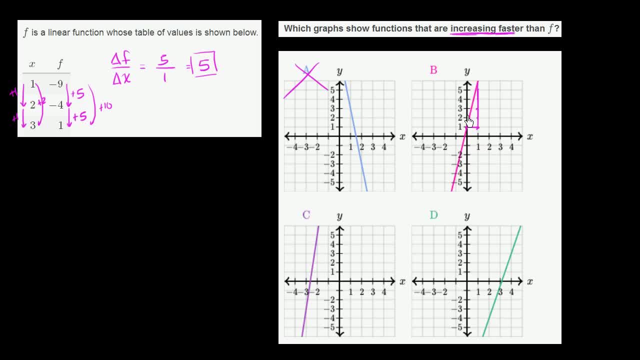 Or our change in y over change in x, is exactly 5.. So it's not increasing faster than f, It's increasing the same as f. Now let's look at c, And so I'm going to try to find a point where it looks like I have kind of an integer point right over here. 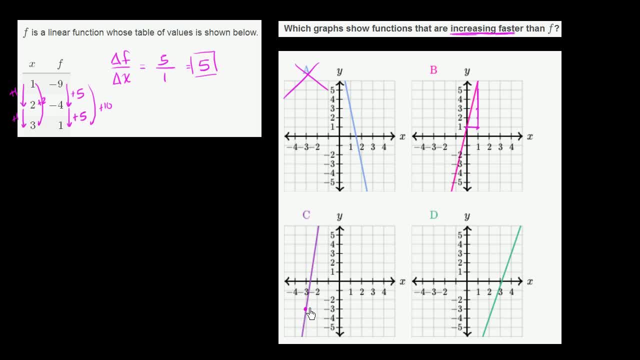 So that's the point: negative 3 comma, negative 3.. And if I move 1 in the x direction, it looks like I'm increasing by more than 5.. I'm increasing 1,, 2,, 3,, 4,, 5,, 6,, 7,, 8, it looks like. 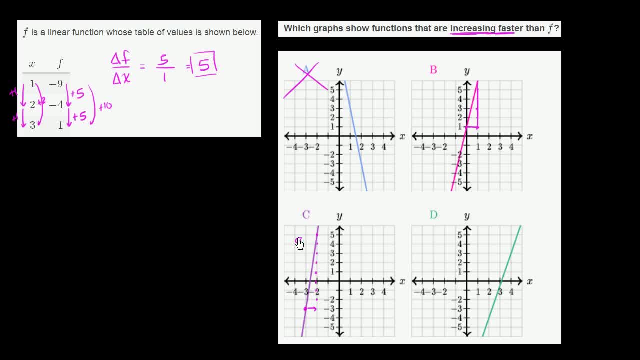 So this one looks like it has a slope of 8. So this one does. this one is increasing faster than f, So we'll circle that right over there, And now let's look at this choice. So if we start right over here and I just 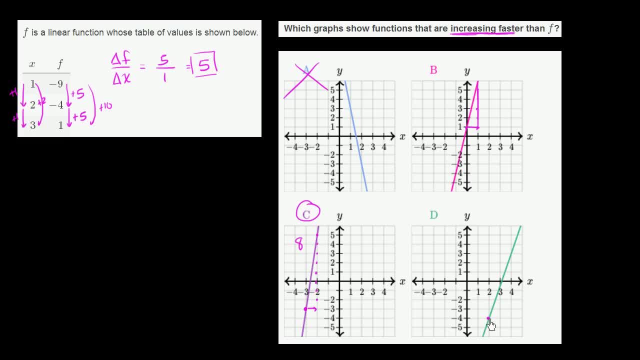 picked this point because that's a nice integer coordinate. It's at the point 2, comma, negative 4.. If we increase by 1, if we increase x by 1, then we increase y by 1,, 2,, 3, looks like about 3 and 1. 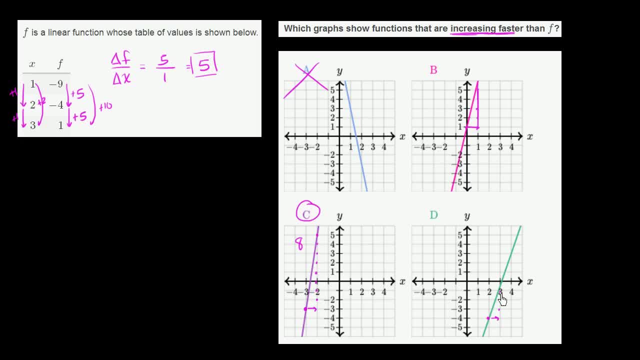 half, definitely not 5.. In order for it to increase as fast as f, it would have to increase by 5. So it would have to be up here. So it would have to go 1,, 2,, 3,, 4,, 5..